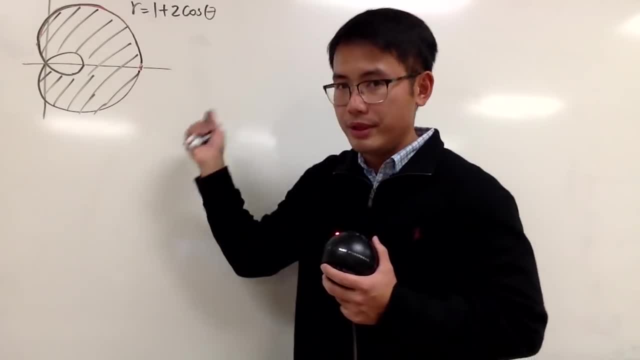 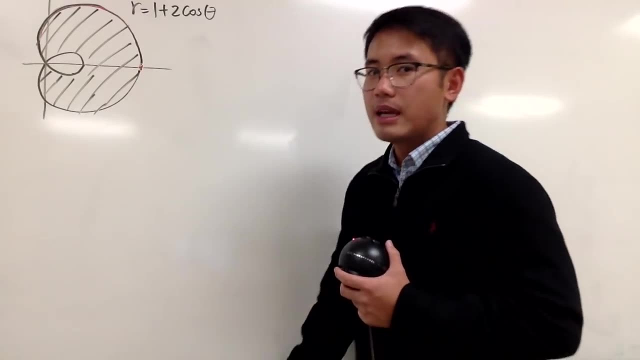 And you'll see that this is actually 0, 3.. 0 for theta r is 3.. That means you are looking at this direction and you are going out 3 units away. And then you can plug in more angle value for theta and you'll actually see that the curve goes like this: 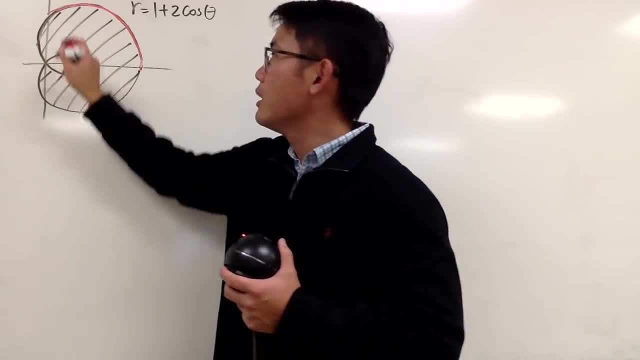 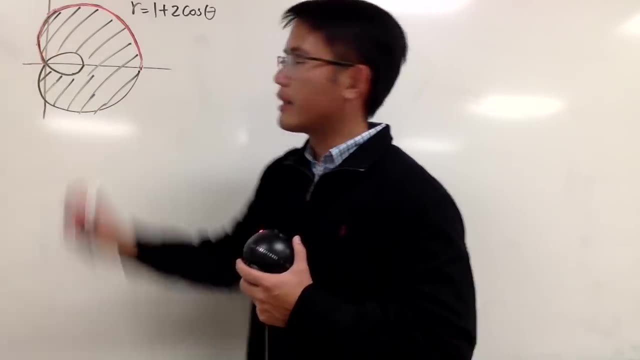 Especially this is when theta is equal to pi over 2, and then it's going to rotate and you are going to get back to the origin like that, And you have to be careful. You have to know for what angle we are going to compare to the origin. 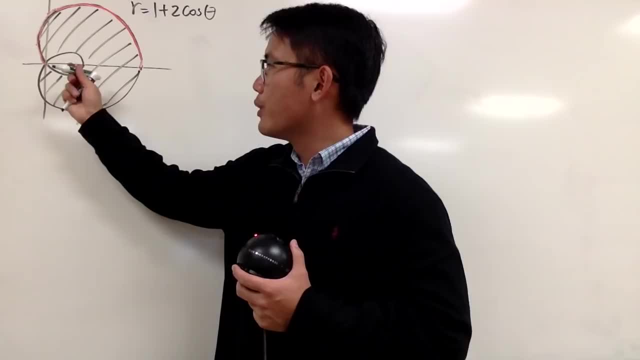 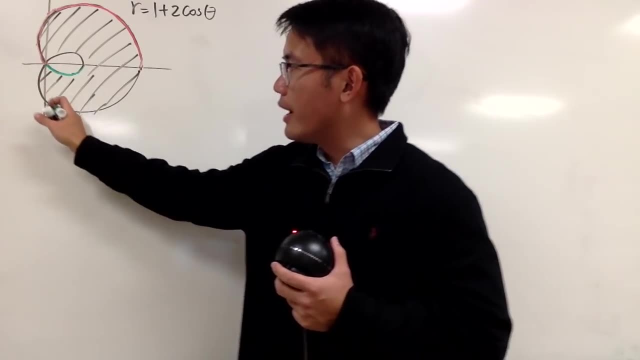 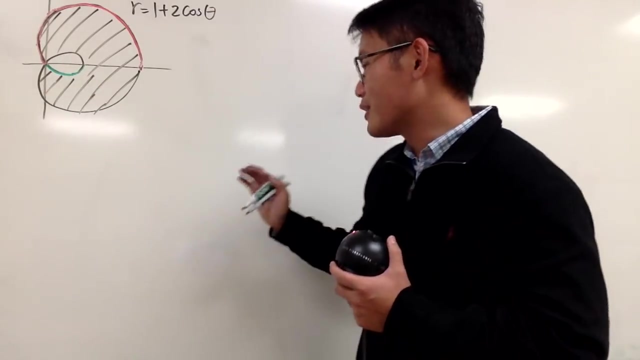 And then after this, we are actually going to go down right here and then it's going to rotate this way and then up, But the good thing is that the area of this part is the same as the area of that part, so it's actually good. 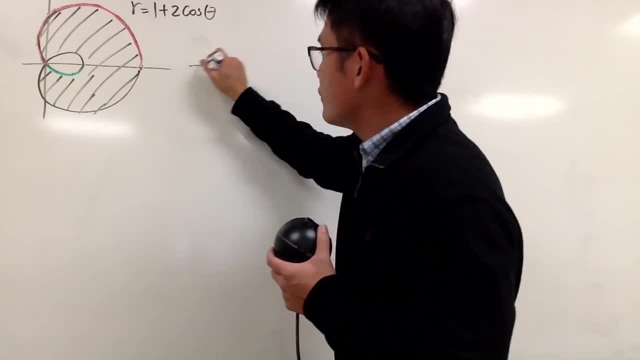 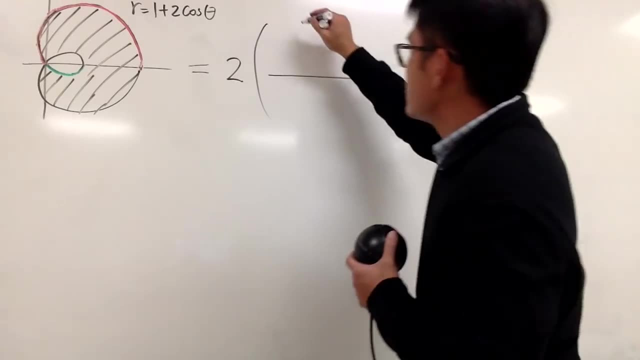 So now let's see. Let me just write this down for you guys, In order for us to calculate this area, I will just do two times the following. The top is this: I go from here and then I rotate to here. 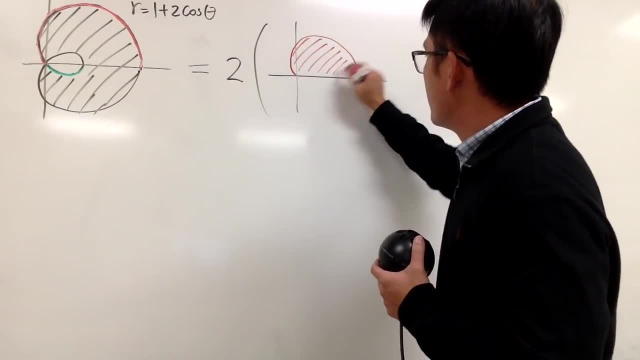 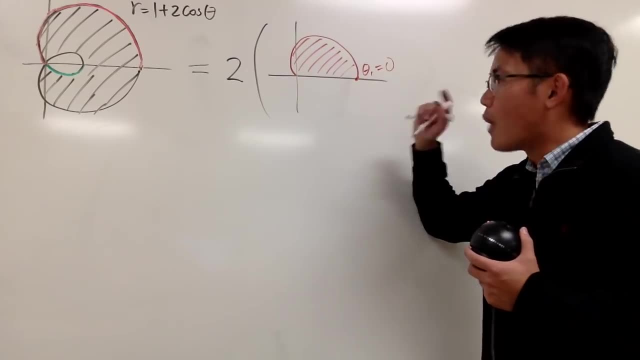 And let's focus on this one first. So let's see, I need two angle values. This right here, as we discussed, it is just 0, and that's my theta 1.. Now for theta 2, it's going to be right here. 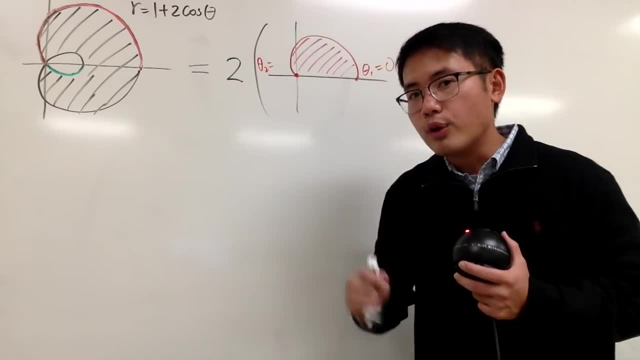 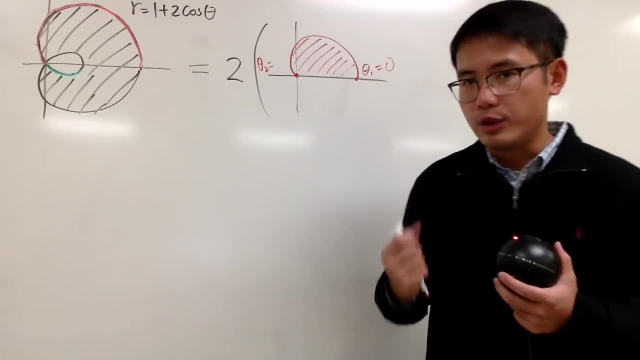 I need to figure out what theta 2 is, And to do so, you have to remember well, at the origin. that's where r is equal to 0 for our polar equation. Therefore, all I have to do is I will just put this down right here. 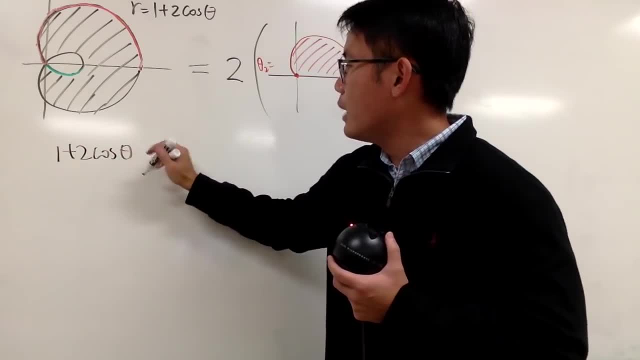 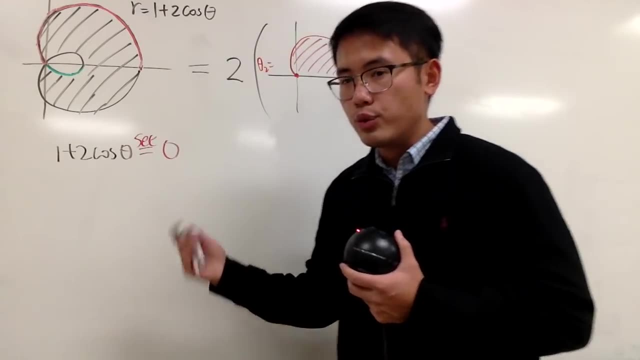 1 plus 2 cosine theta, I will have to set this to be 0. For the origin. And then of course we can just solve this equation real quick. We can minus 1 on both sides and then divide it by 2 on both sides. 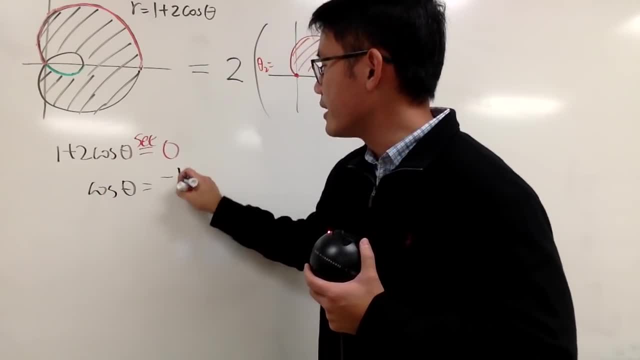 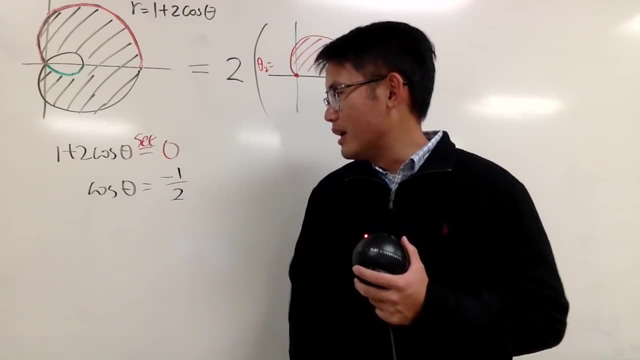 So we see that we have cosine theta is equal to negative 1 half. And from here, depending on how you want to solve this equation, you can just recall your cosine values at different angles, But you can also draw reference triangles. I will do that for you guys. 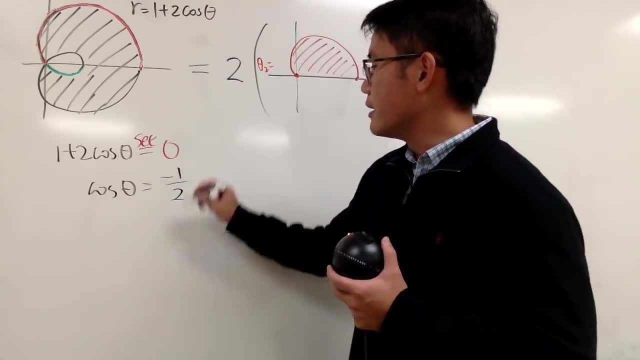 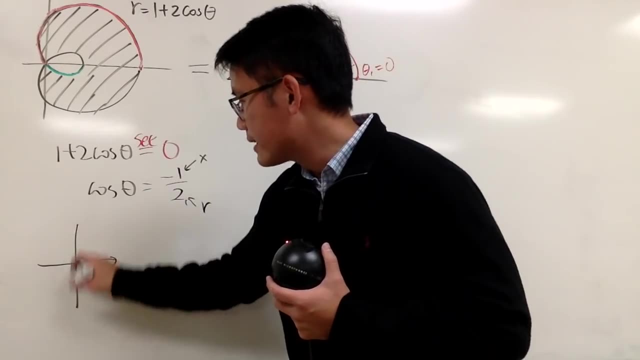 To draw the reference triangle. you have to remember cosine is x Over r And what I mean by that is you can look back to your x and y plane. When x is negative 1, it's right here. Right Next, negative 1 is right here. 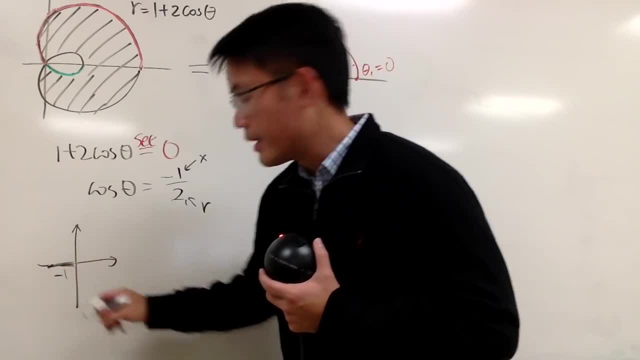 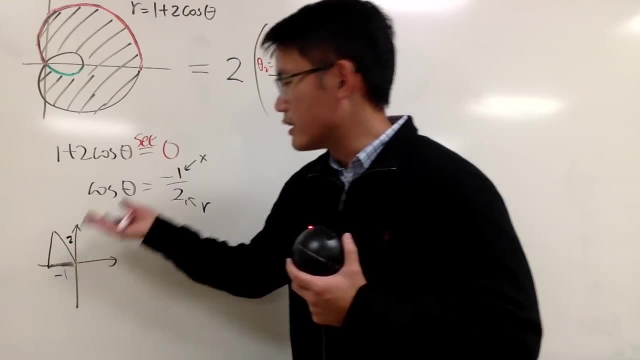 Change the market. This is negative. 1. You have to go to the left And then r is 2. Then you just go from the origin, 2. Like this, And this is a special right triangle, because we have negative 1,, 2, and this right here will be square root of 3.. 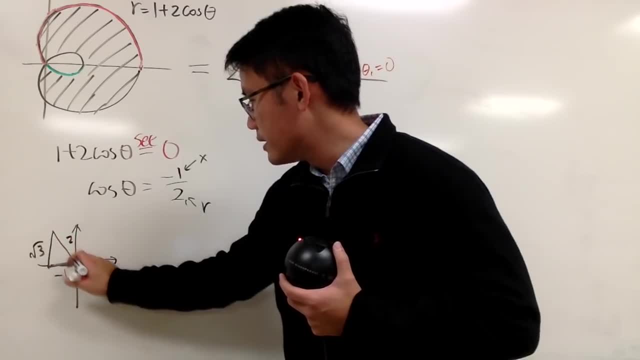 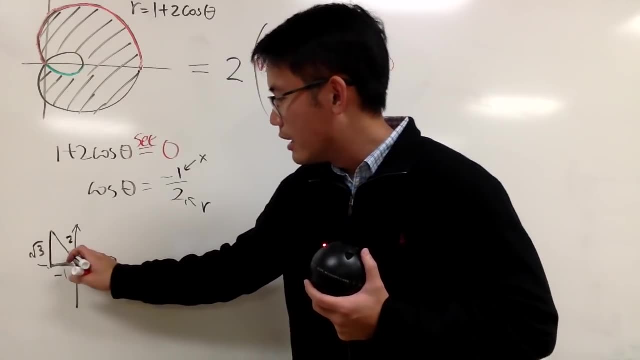 So you have to know that this is actually going to be a 30,, 60,, 90 special right triangle And this is going to be 60 degrees Inside. well, that's the same as pi over 3. 60 degrees. 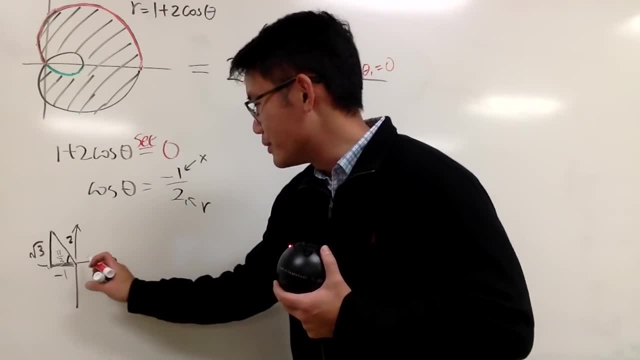 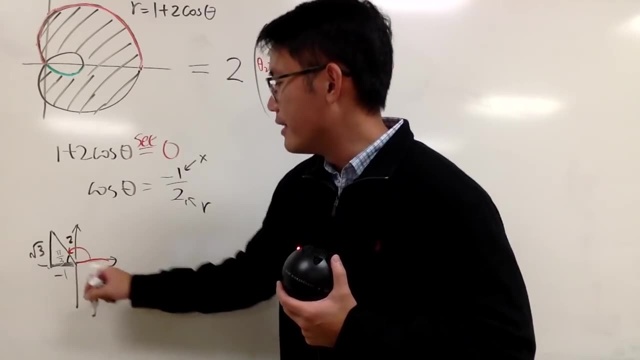 Well, you don't look at pi over 3.. You need the angle from the positive x-axis to here, And of course this angle is just pi minus pi over 3. And that will give us 2 pi over 3.. 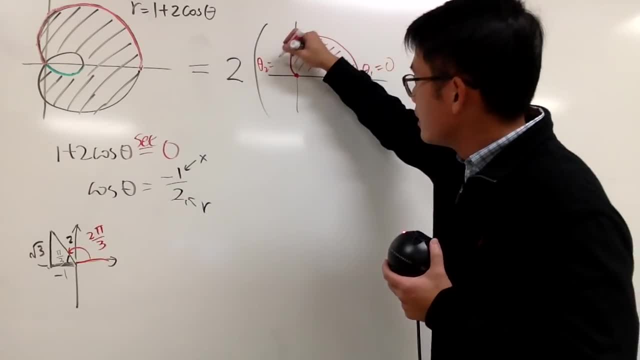 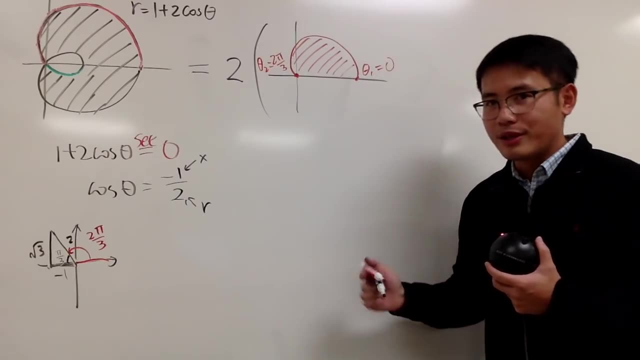 And that's precisely the theta 2 that we need. Let me just write down 2 pi over 3.. And there you have it. Once you have the angle 1 and angle 2, this right here is actually pretty easy now. 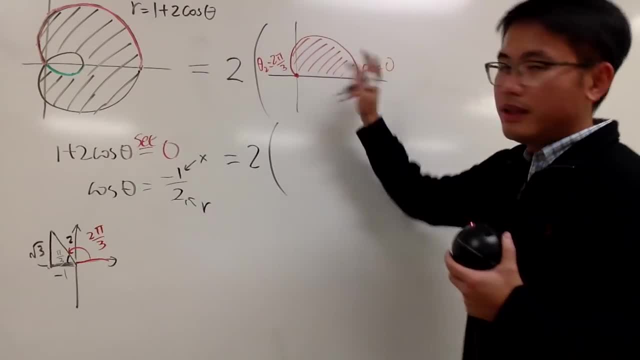 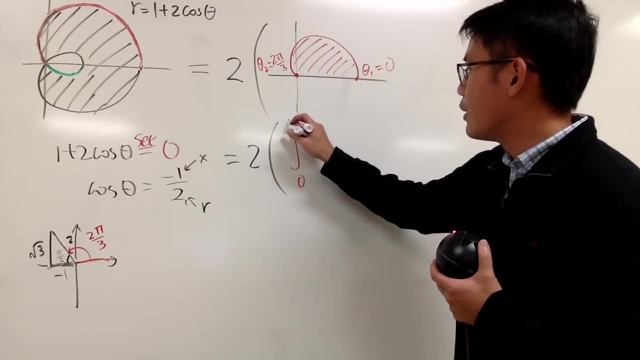 So don't forget the 2 all the way in the front. And for this area I will just put down the integral in red. We go from 0 to 2, pi over 3.. And then, remember, the formula is 1: half. 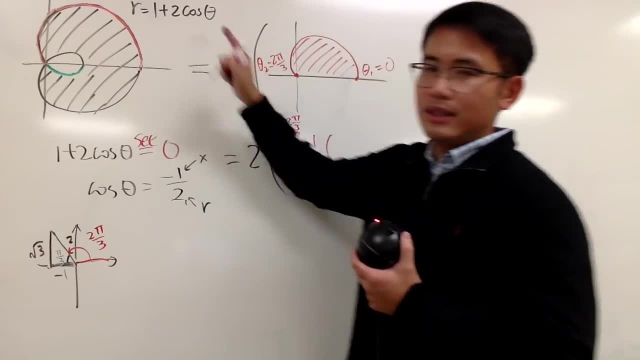 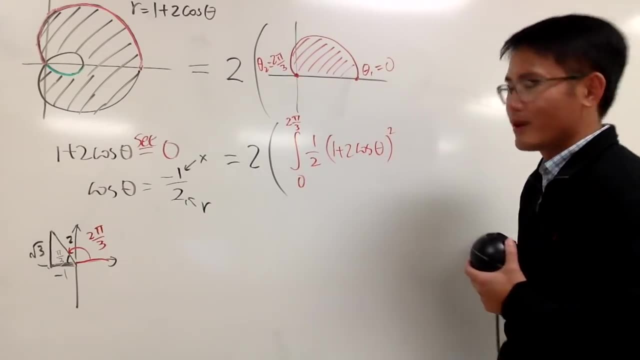 times r squared, And r is this. So you just going to enter that into the parentheses: 1 plus 2 cosine theta, And then don't forget the square, And then, of course, d theta. This will calculate the area, right here. 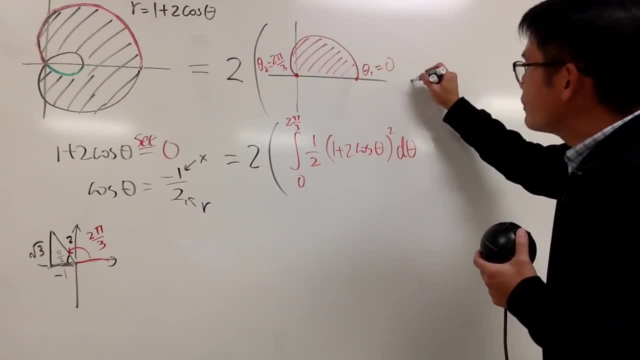 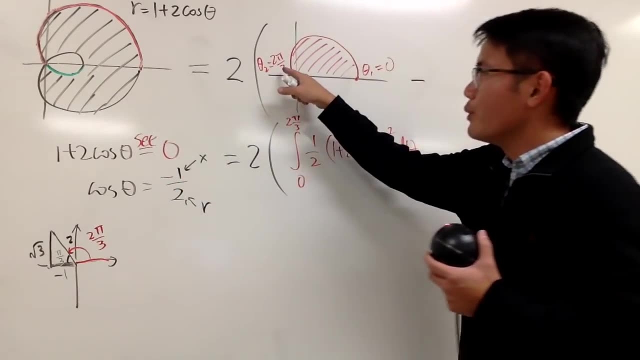 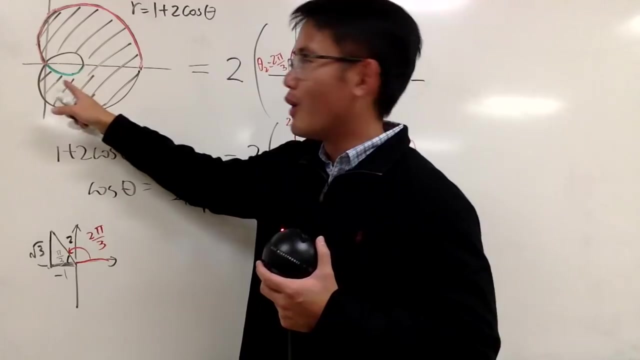 Now the second part is that we have to subtract- And I should be subtracting this, But if you want to continue, the angle value from 2 pi over 3.. From 2 pi over 3 to the next value is actually right here, So I will. 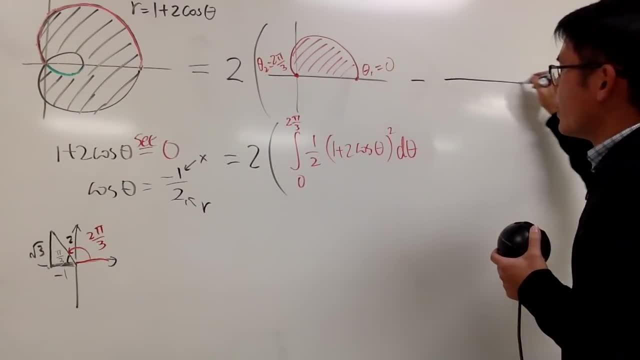 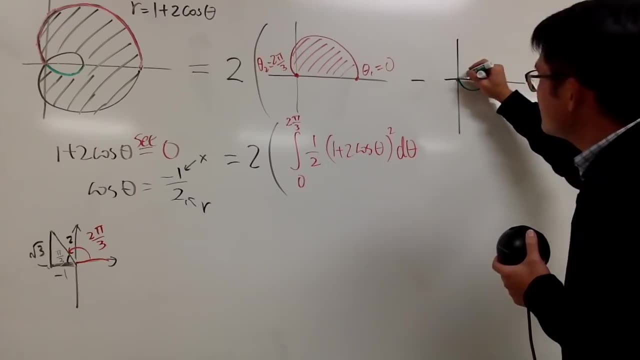 just draw the bottom portion for you guys. It's the same. anyway, The bottom and bottom are symmetrical. They are nice people. Anyway, from here to here, What is this angle? Well, this is my starting angle this time. That will be my theta 1, which is, of course, 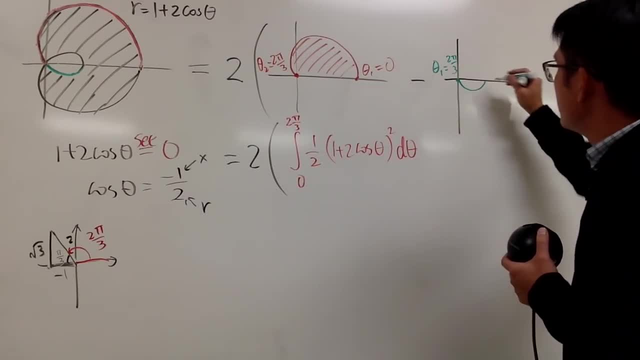 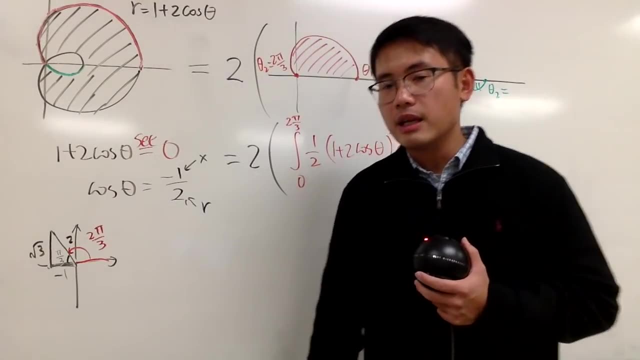 the same as that 2 pi over 3.. That's nice. Now, what is this angle, though? This is going to be my theta 2. So a small tip for you guys, Anytime that you are on the x axis. 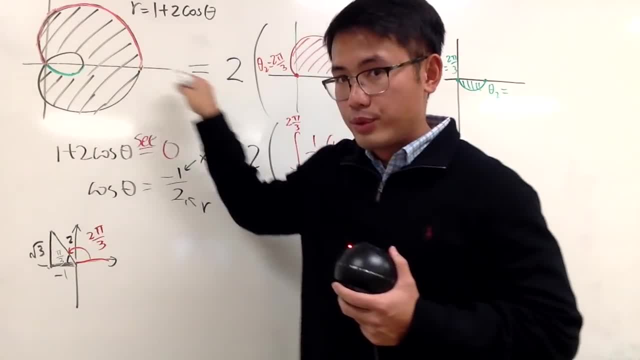 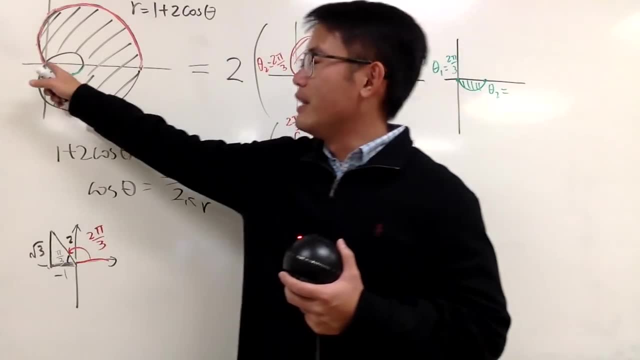 you are going to be having either 0 or pi, or 2 pi or any multiples of pi. Okay, Except for at the origin. At the origin, you have to figure it out by setting the r equal to 0.. But, of course, right here, 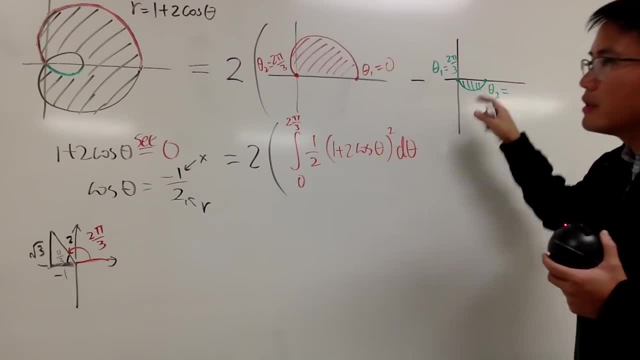 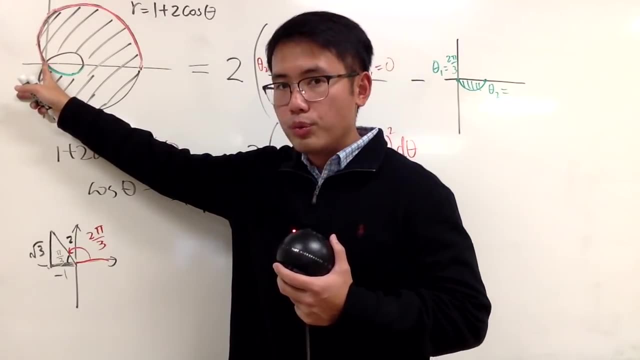 you can just think that it's on the x axis. So it's either 0, pi, 2 pi and so on. And you see, earlier we went from 2 pi over 3 to actually pi. So theta 2 right here is actually. 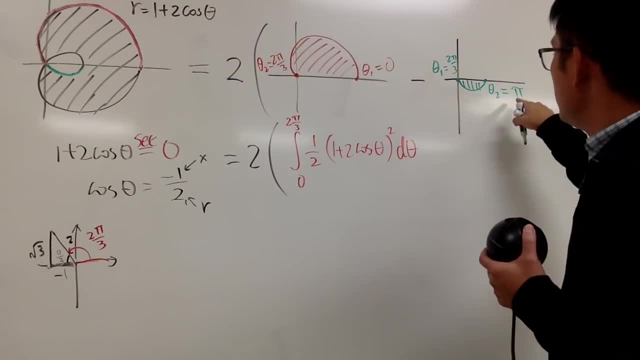 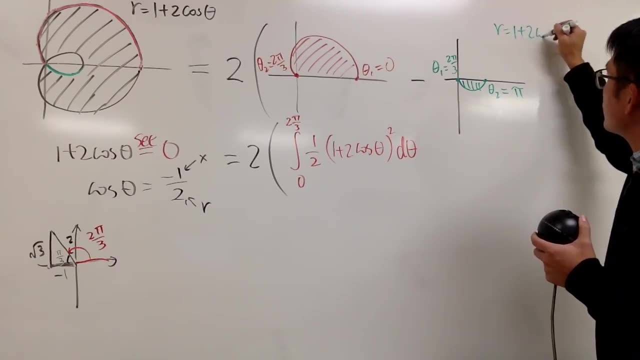 pi. It's kind of weird, but I'll show you why. If you plug in pi into the equation, you get r equals 1 plus 2 cosine pi. Cosine pi is negative 1.. 2 times negative 1 is negative. 2 plus 1,. 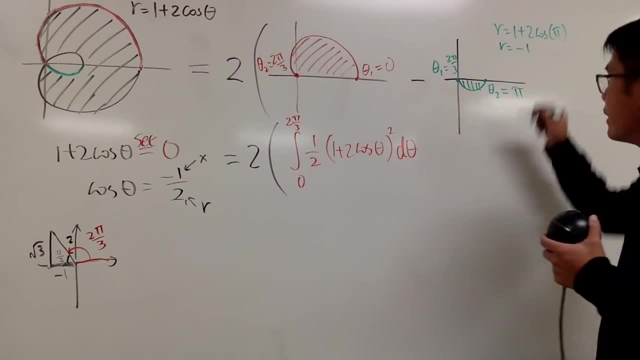 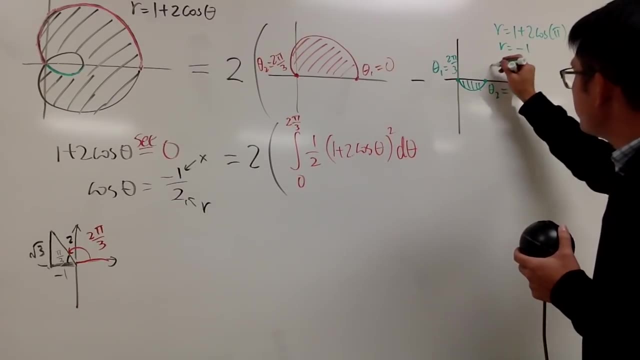 so r is equal to negative 1.. So this point is saying you have pi and negative 1 right here, right, And for the polar coordinate you have to write it as negative 1, for r and theta right here. So this is r. 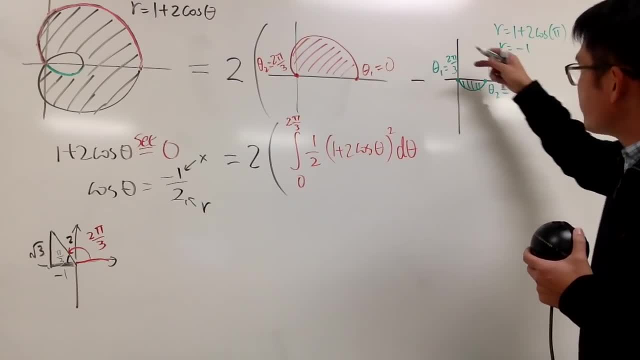 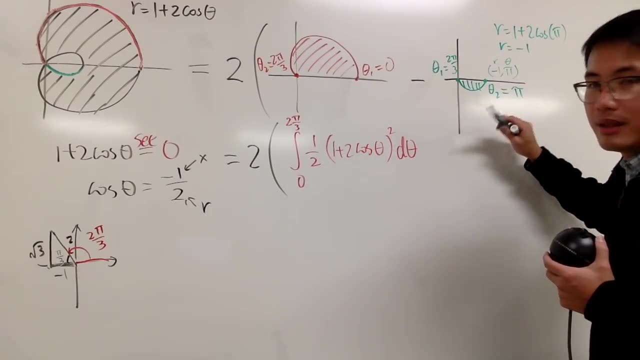 theta, And this means you're looking at the pi direction which is over there. that direction, r, is negative 1.. That tells you to go back one unit. So you are looking at that direction and move back one unit. so you are. 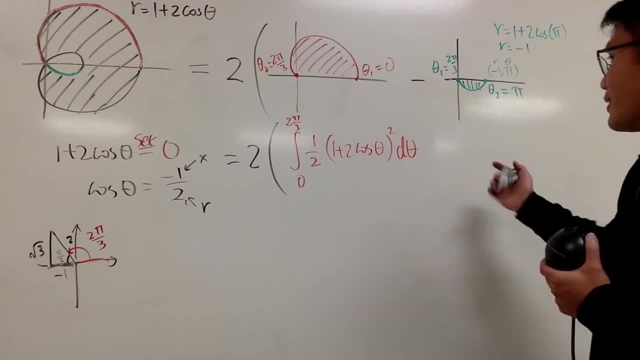 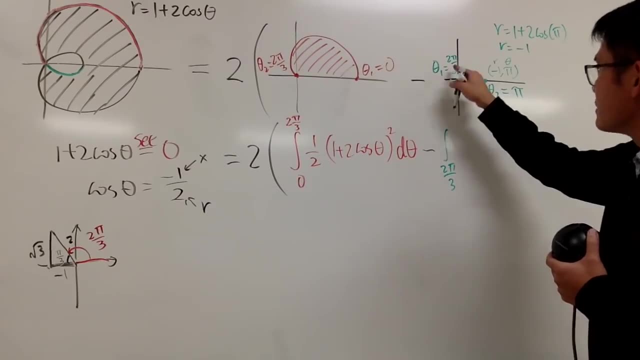 right here at this point. So that's pretty much it. So the good thing is that we are pretty much done. I can just subtract the integral from 2 pi over 3, that's my theta 1 here and then to pi.